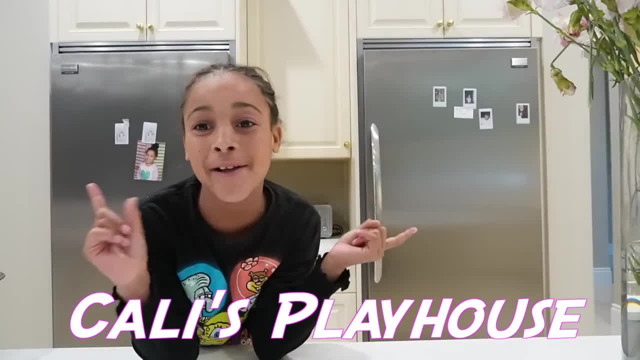 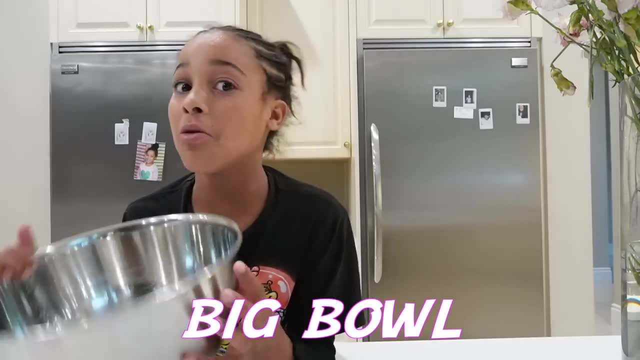 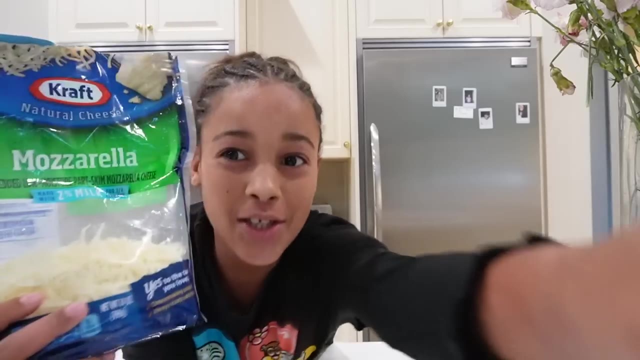 Hi guys, welcome back to Callie's Playhouse. and today we are going to be making a salad in this big bowl. So I guess the first step is a big bowl. if you're making a big salad, The ingredients are some mozzarella cheese, cucumber, lettuce and carrots and ranch for. 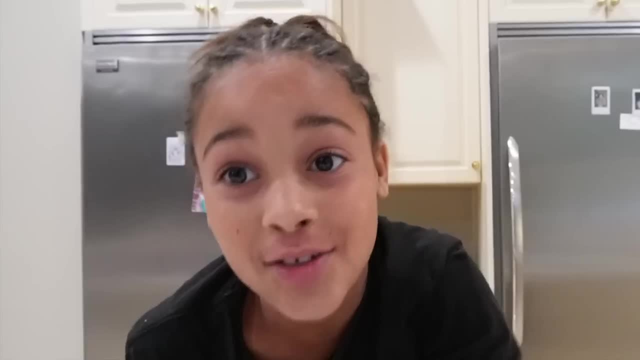 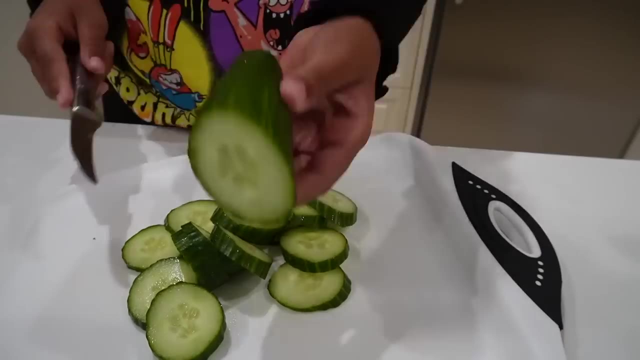 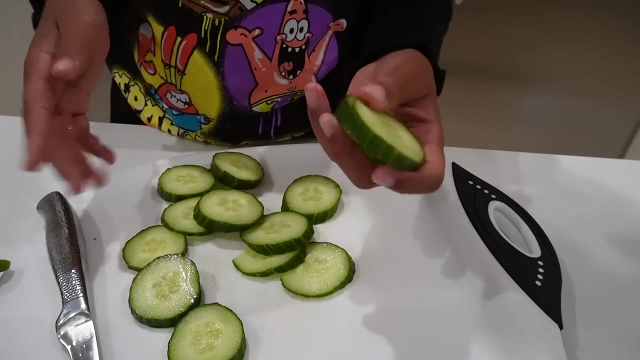 sure, Now I'm going to start cutting stuff up. Don't worry, it's a soft knife, so I'm not going to cut myself. So now I cut it in these pieces, but now I'm going to cut it in like small square shaped pieces. So yeah, 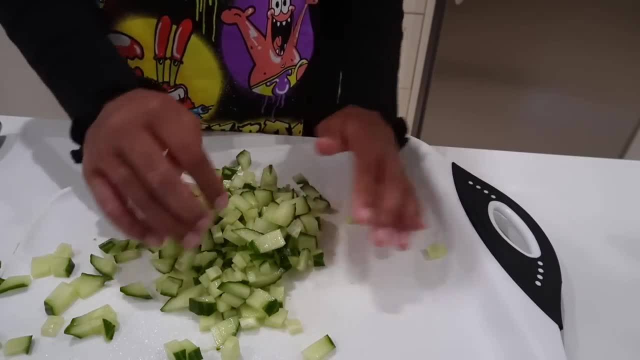 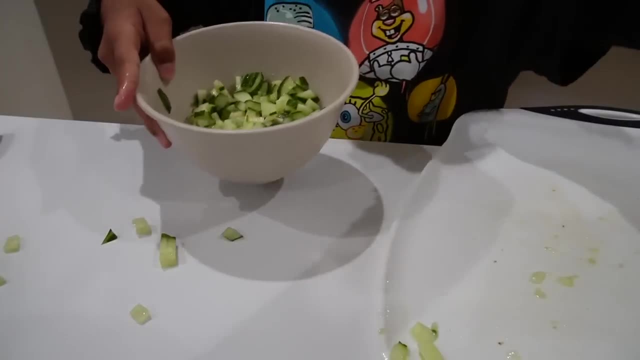 All right, so I just cut it in half. All right, so I just cut it in half. All right, so I just finished cutting up all of the cucumber and let's move on to the next item. Oh yeah, Next is carrots. 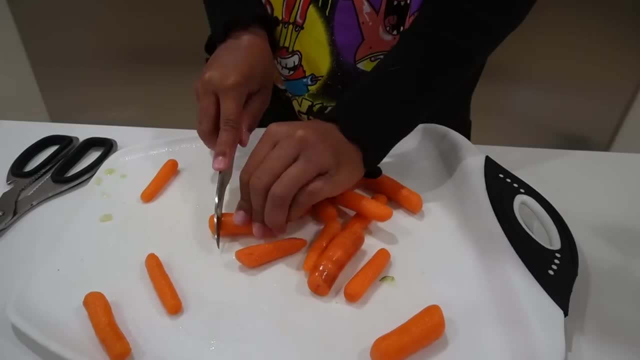 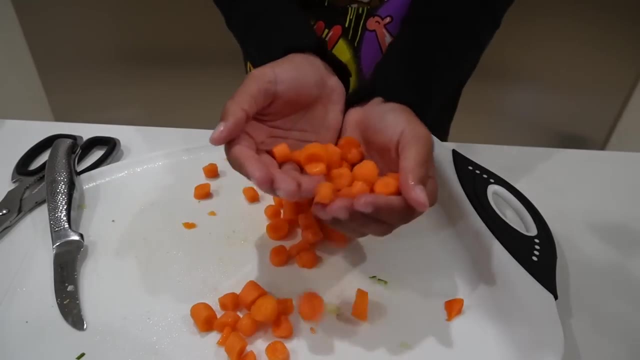 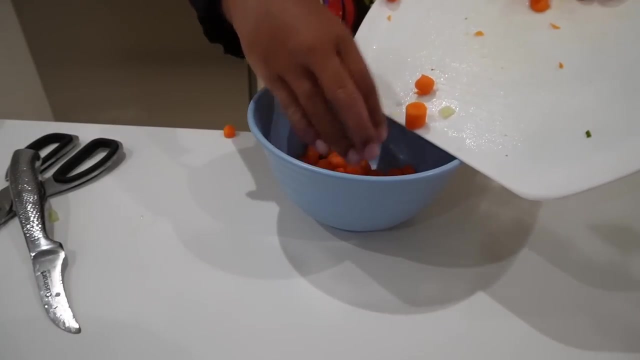 I know I think this is too much carrots, but we're going to do it. I am all done with these carrots, So now let's put them in the bowl. Time to put these carrots in the bowl, And it looks like the carrots are. I believe I can fly. 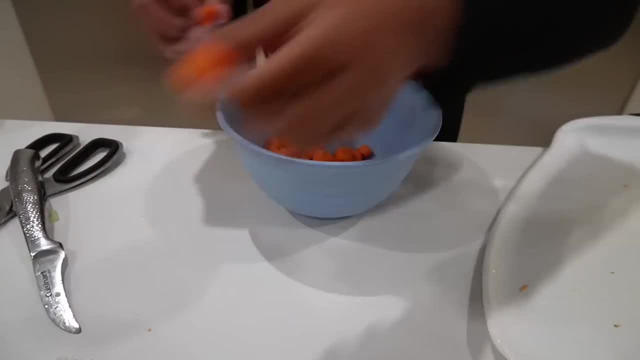 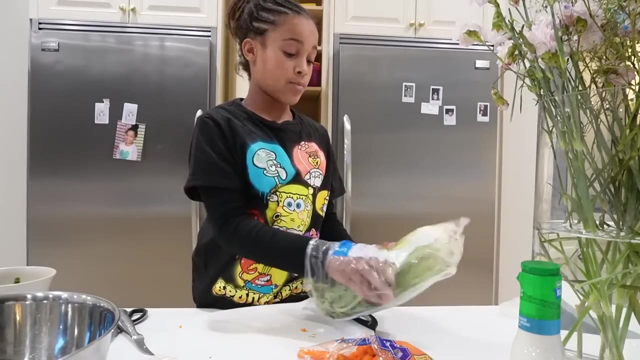 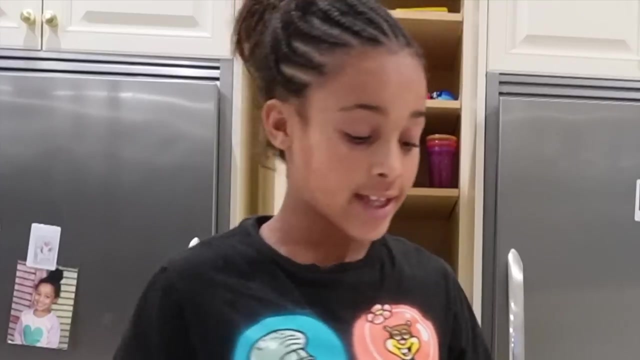 I believe I can touch the sky, But they're not touching the sky today. Here are the carrots. It's time for the lettuce. All right, so I'm going to start cutting up some lettuce. So I'm just going to cut off the ends first, and then I'm going to wash it. 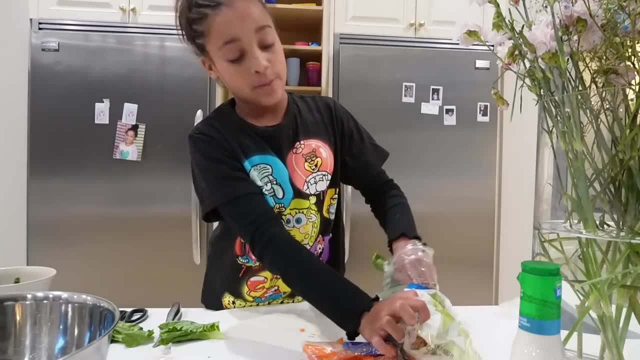 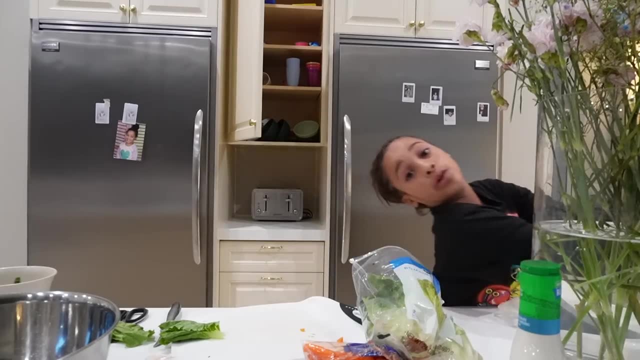 This is not going well with like these lettuce pieces coming off, so I have to get it. it just fell on the floor, so that's how you know. I'm just gonna wash this one quickly. Okay, that's better. So let me just cut off the ends. 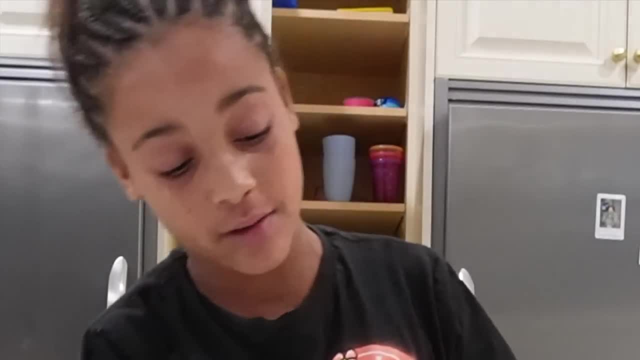 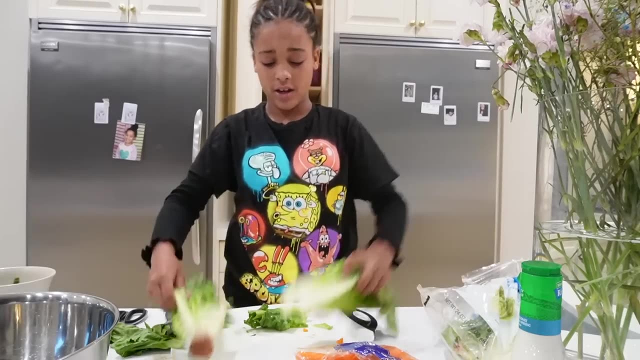 because it doesn't look like the ends are doing too well. We need a lot of lettuce, because let's just get this whole thing- because we're making a lot of salad right now- Cut off the end. it's a whole mess in here. 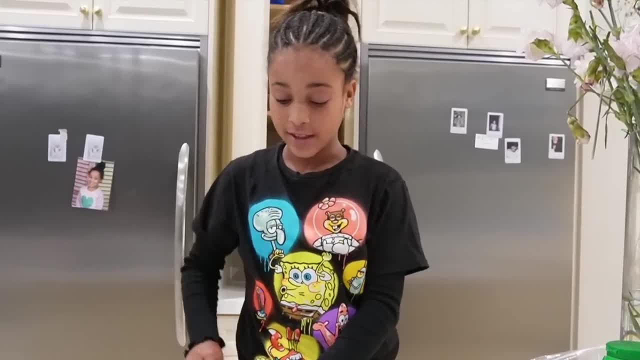 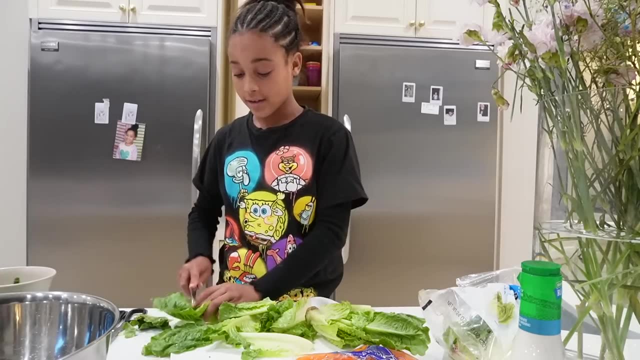 This piece is okay. Lettuce is like pretty much a leaf. Well, I guess lettuce is a leaf Cut off the ends. but the ends that are not bad, we'll keep them. So that looks like enough lettuce. Now it's time to wash them. 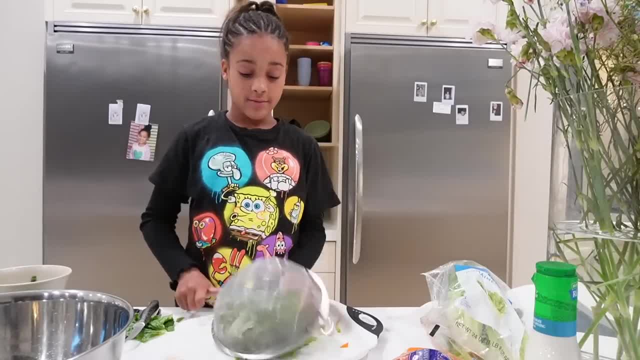 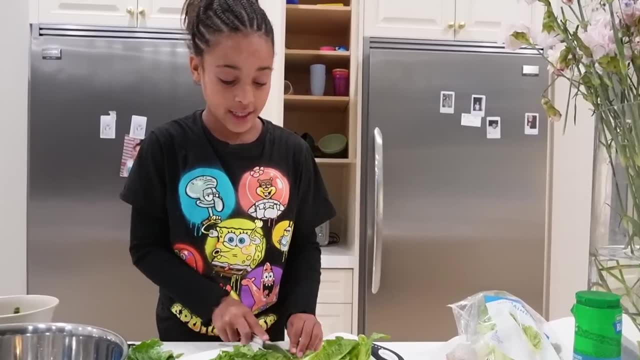 Okay, I just finished washing it, So now I'm just gonna plop the lettuce in there. And now let's start chopping. It's not that hard to really cut lettuce. You just need to cut it in like those, like pieces. 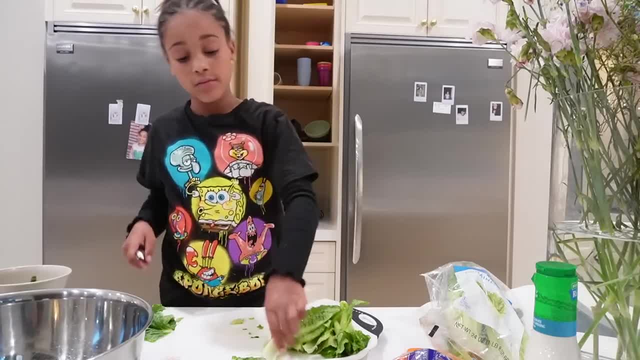 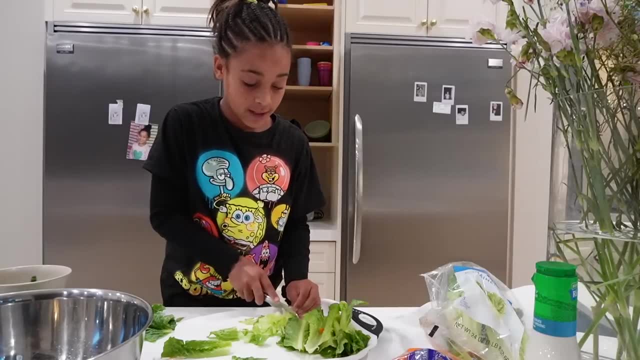 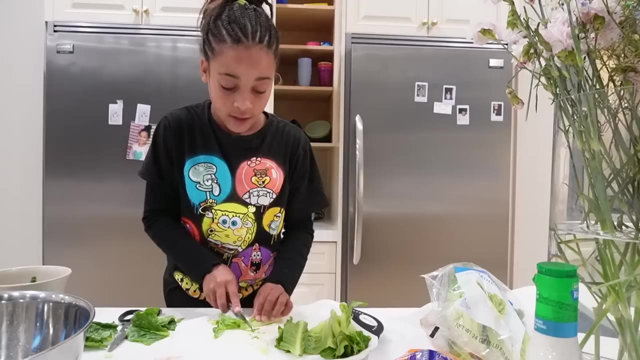 Plop it in our bowl. Plop. And now let's do our next one. Just cut Like it's not even hard. Cut, cut, cut, Cut. Plop it in your bowl. Just keep on doing that over and over and over again. 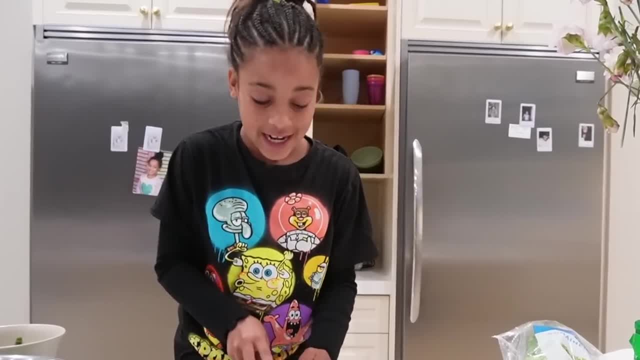 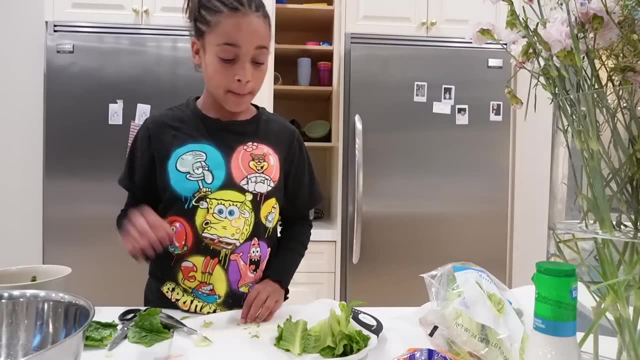 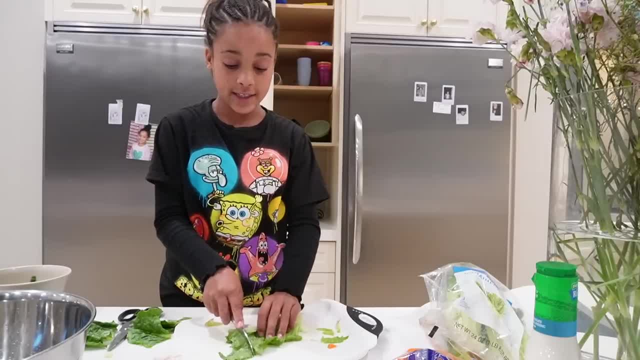 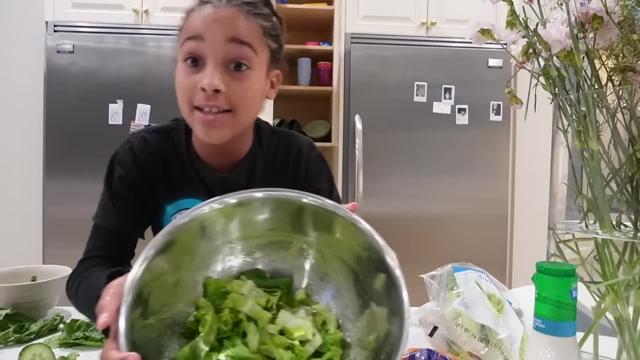 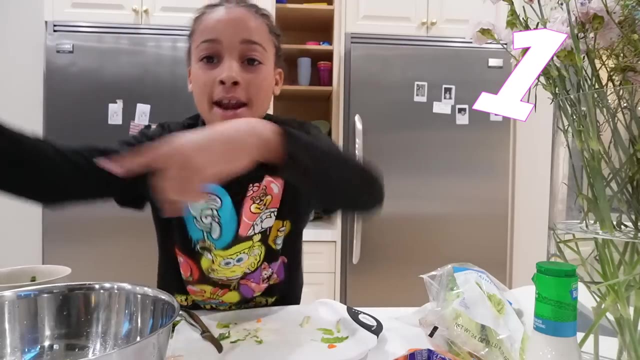 but that's okay. It's actually kind of fun cutting lettuce, Cause it just one, two, three, four, five, six, seven And this is not enough. So we need to get more lettuce. And three, two, one. 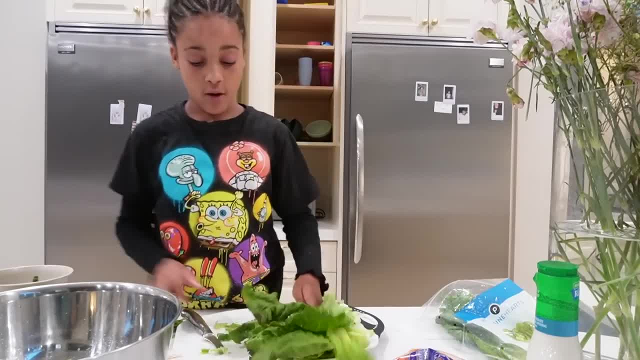 Boom, Just finished washing the other half And now I'm gonna start cutting off the ends. And now I'm gonna start cutting off the ends. And now I'm gonna start cutting off the ends And putting them on the table to make a mess. 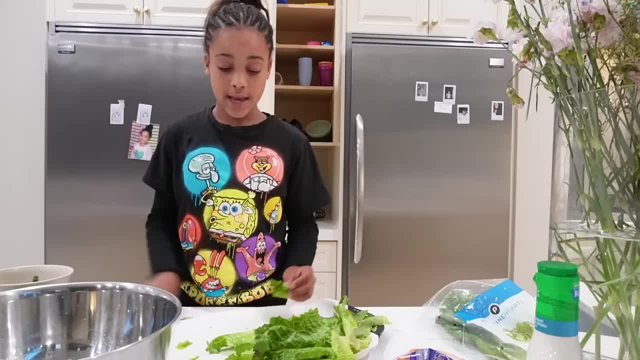 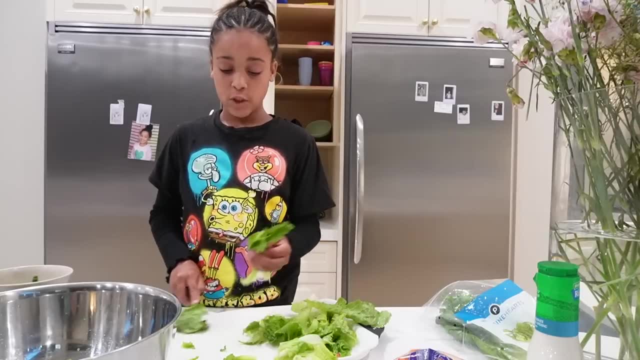 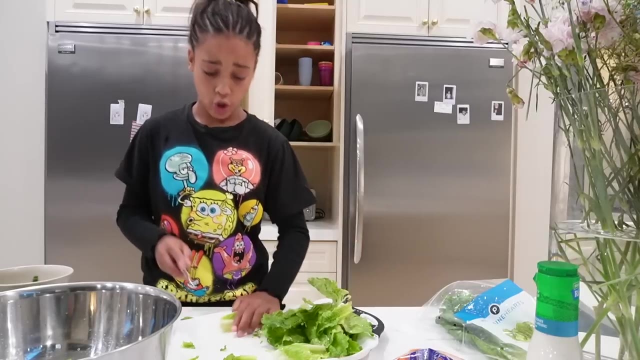 And yes, it's like kind of a mess Snip and then we throw it to the side. If it has a bad end then it will just snip off. That lettuce went flying, Now. that's good. So now we're gonna start snapping. 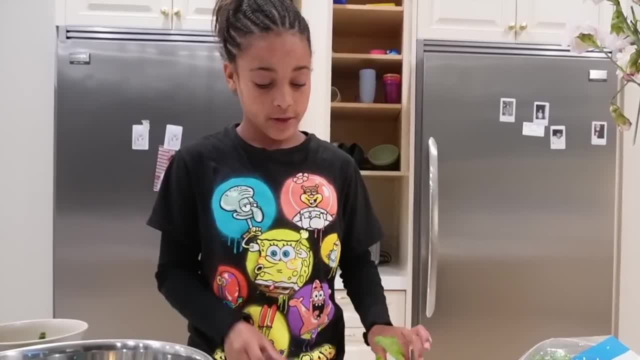 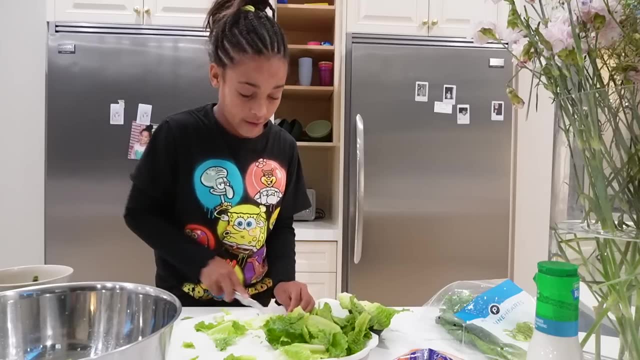 One, two, three, four- Did four on that- And plop it in your bowl. And plop it in your bowl: One, two, three, four, five, six, seven. Plop it in your bowl. Now I'm gonna start doing two at once. 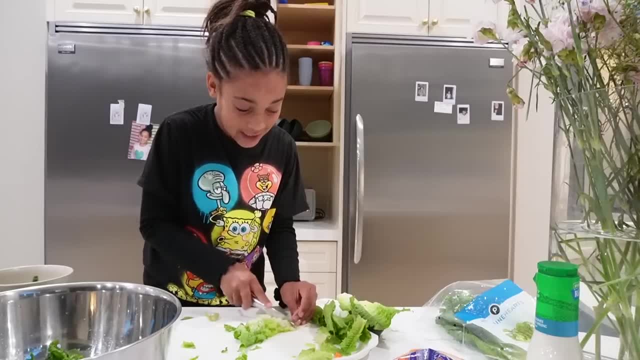 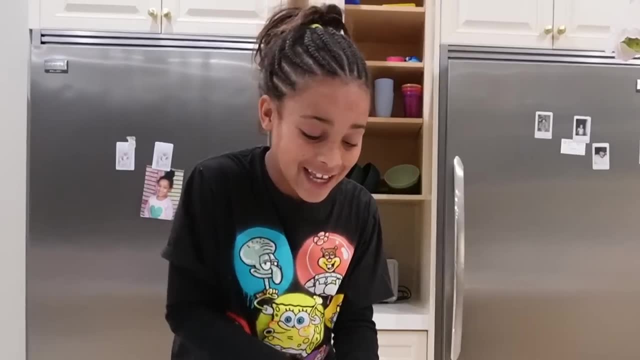 One, two, three, four, five, six, seven. Let's see if we can get to eight. One, two, three, four, five, six, seven, eight, Not ten, Not ten Dang. I still don't know if that's enough lettuce. 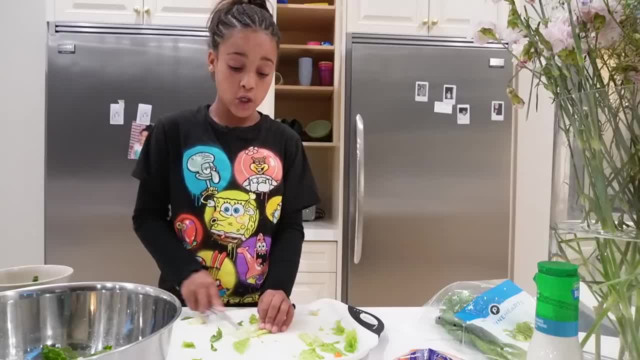 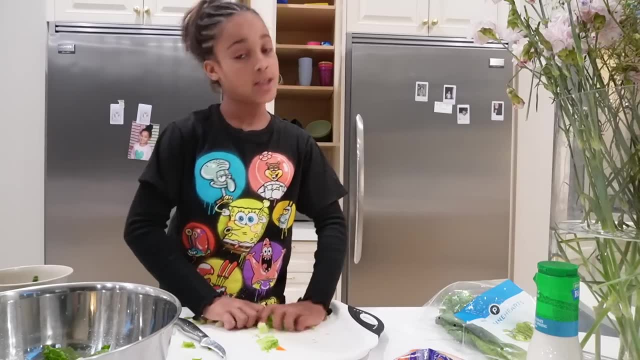 So I think I'm just gonna get a little bit more. So I think I'm just gonna get a little bit more, But first just need to cut this up a little bit And this And plop it. You heard it, plop it. 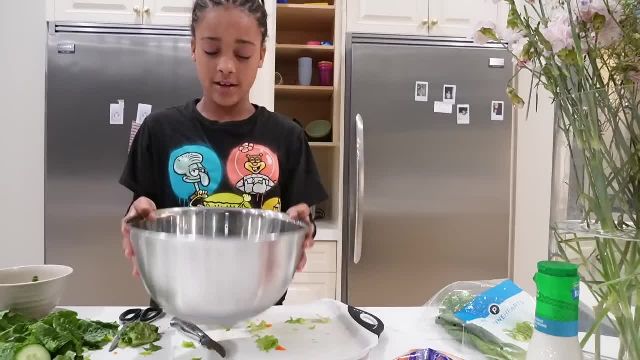 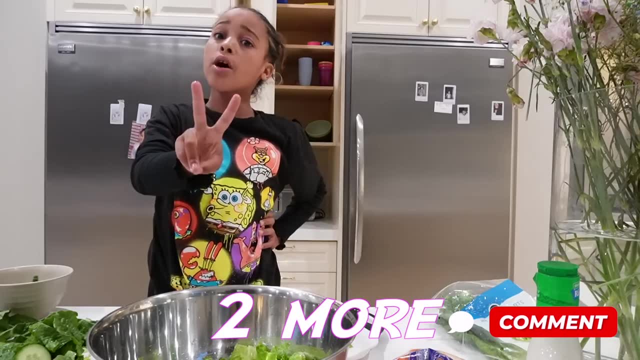 That's how much we have. I don't know if it's a, if it's enough lettuce. Hmm, do you guys think this is enough lettuce? I think we just need like two more. So let's get two more lettuces and let's finish it up. 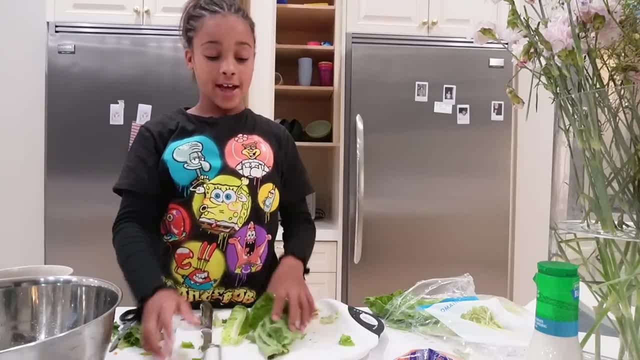 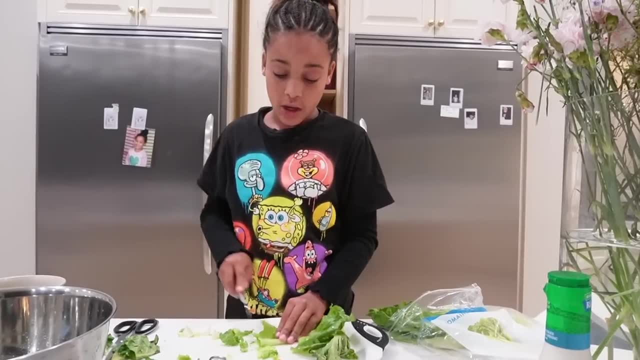 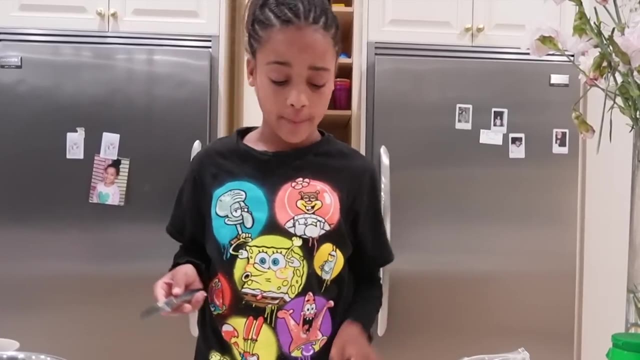 Three, two, one. All right, I actually got three out. So now we're just gonna start chomping: One, two, three, four, five, six, seven, eight, nine, 10.. Ooh, we got 10 chops on that. 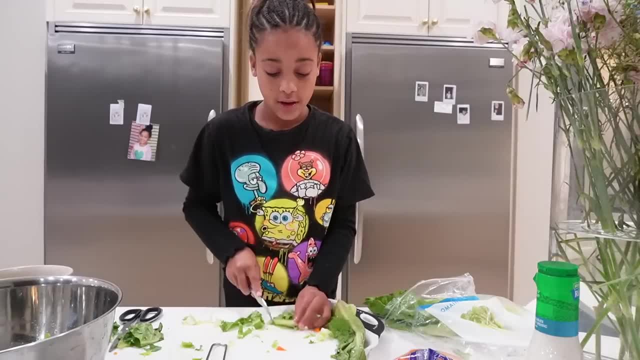 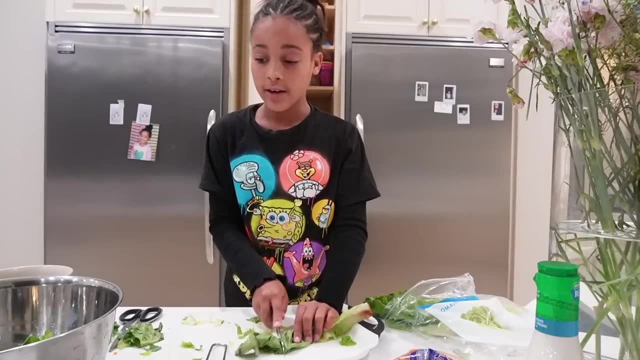 Let's see if we can get 11.. One, two, three, four, five, six. That was six. That was a small one, And now we got our last one And let's count: One, two, three, four, five, six. 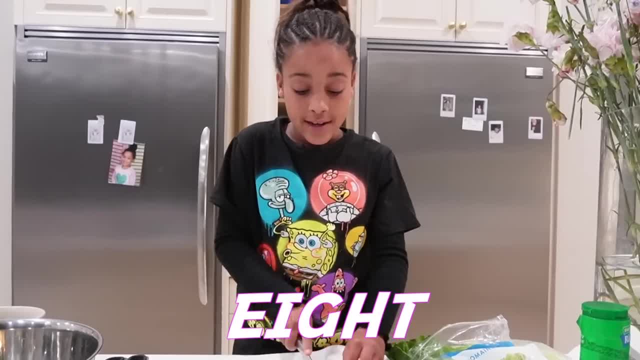 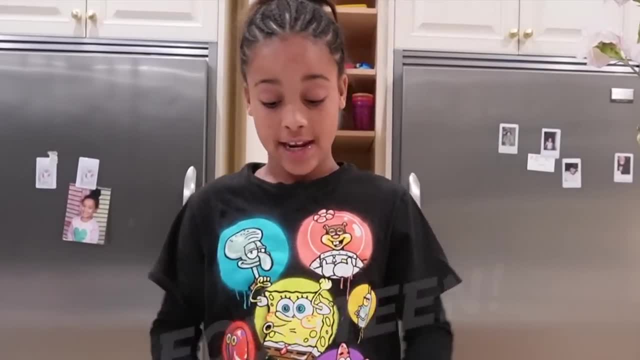 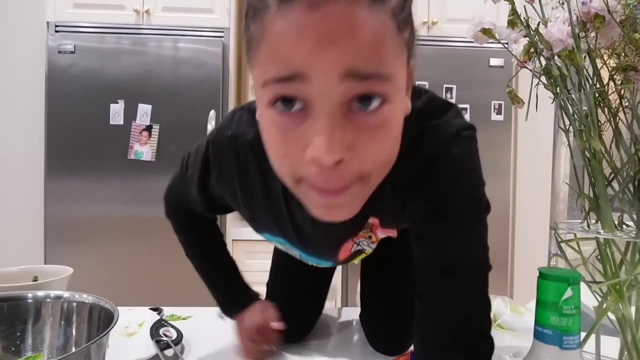 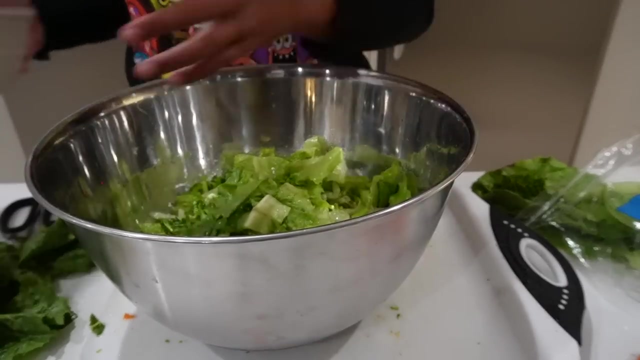 Seven, eight, nine, 10,, 11,, 12,, 13,, 14.. And now we got enough lettuce to make our salad, And I'm gonna have to just cut the clip real quick. Here is our salad. So we're gonna start by adding our cucumber. 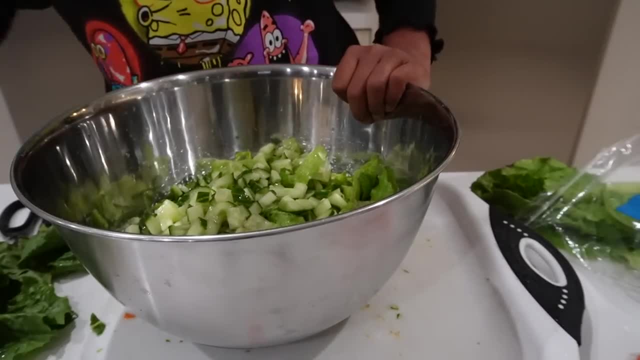 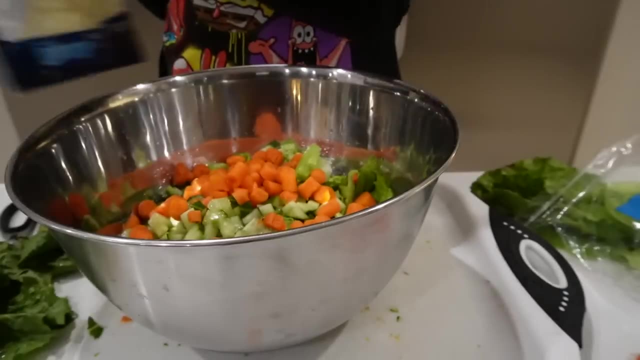 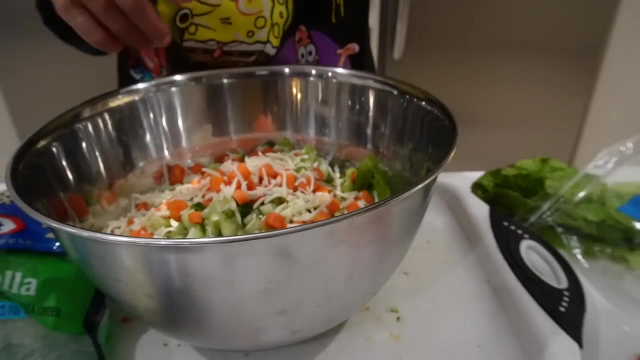 Better cucumber, Better cucumber. Some brim. Now we're gonna get some carrot. Now we're gonna put some mozzarella cheese in here. Let's put a little bit more. Okay, that was good. Now we're just gonna shake it up like this: